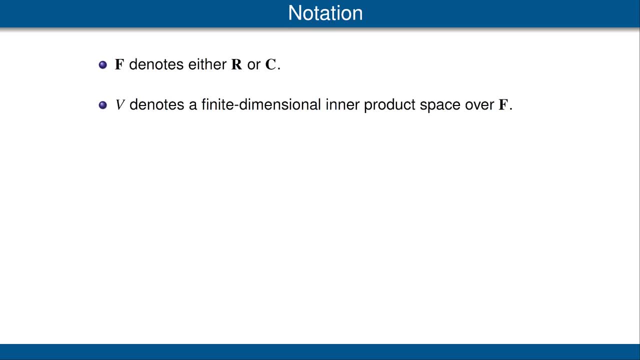 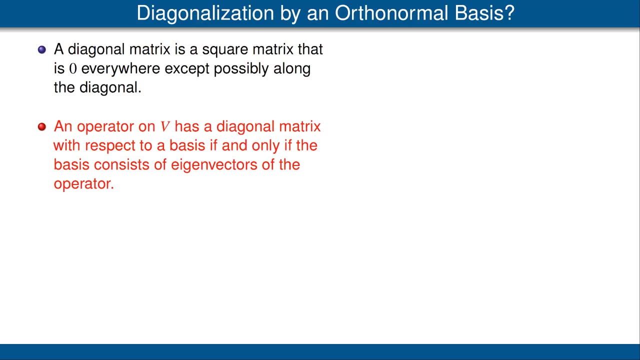 let V denote a finite-dimensional inner product space over F. Recall from a previous video that a diagonal matrix is a square matrix that is zero everywhere except possibly along the diagonal. Also recall an easy theorem that we discussed: Suppose we have an operator on V and a basis of V, Then the matrix of that operator with 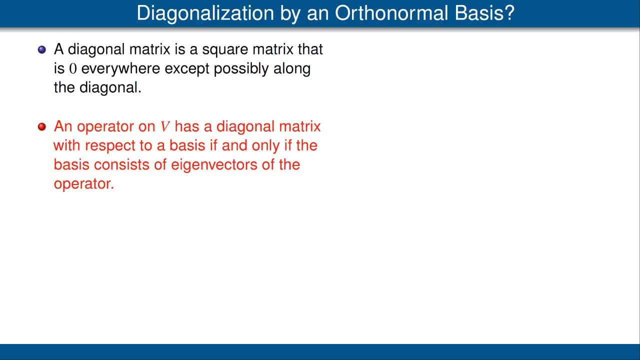 respect to that basis is a diagonal matrix if, and only if, the basis consists of eigenvectors of the operator. You should pause the video and review that result until you thoroughly understand it, because we will need it in what is to come. Because we are working on an inner product space, we should ask not only for a basis. 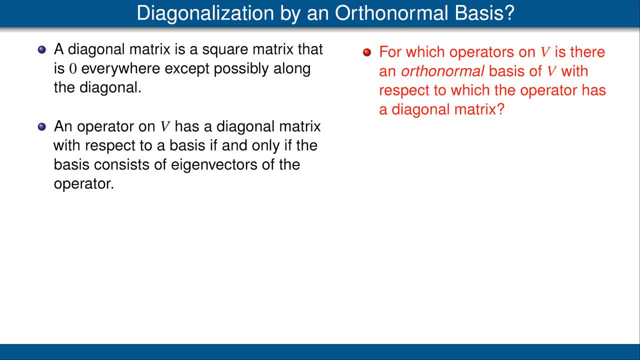 with respect to which an operator has a diagonal matrix, but something even better: For which operators on our inner product space V, is there an orthographic matrix For those operators? we have the best possible description of them Because of the result in the last bullet point of the left column this question is equivalent. 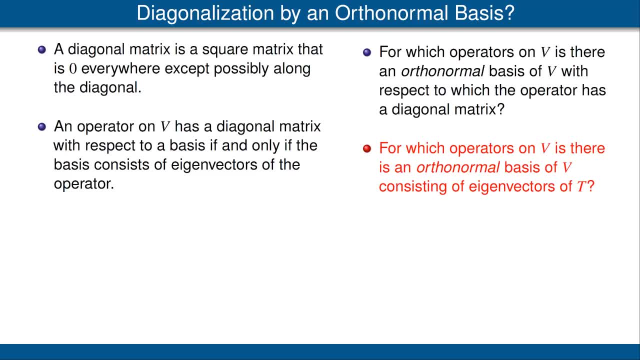 to the following question: For which operators on V is there an orthonormal basis of V consisting of eigenvectors of T? As we will see, the result called the spectral theorem will answer both these questions. The answer actually depends upon whether the scalar field is real or complex. Thus we 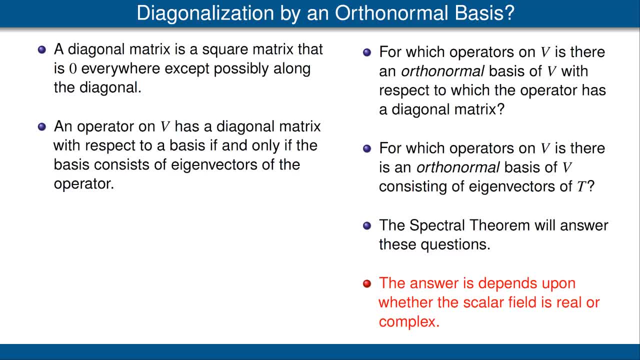 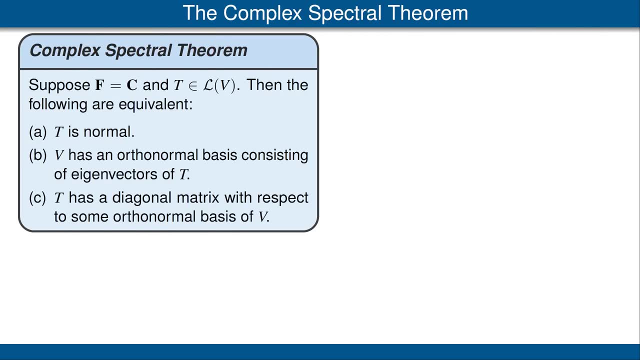 will separate the spectral theorem into two parts, called the complex spectral theorem and the real spectral theorem. The complex spectral theorem is actually a bit simpler than the real spectral theorem, at least in its proof. Thus we will deal with the complex spectral theorem first. 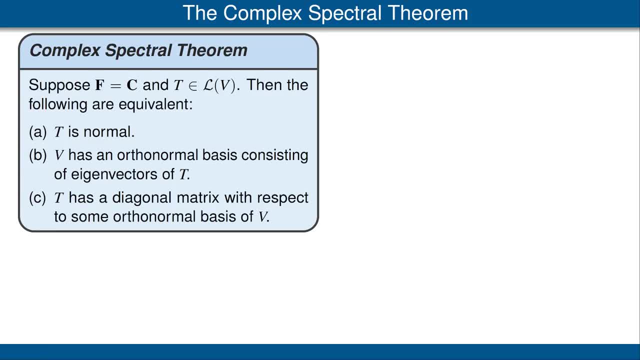 The complex spectral theorem is one of the most important theorem in the universe. In one example, the complex spectrum theorem is actually one of theorems in linear algebra. Thus it deserves a bit of Beethoven's victory music. The complex spectral theorem states the following: Suppose we have a finite-dimensional complex. 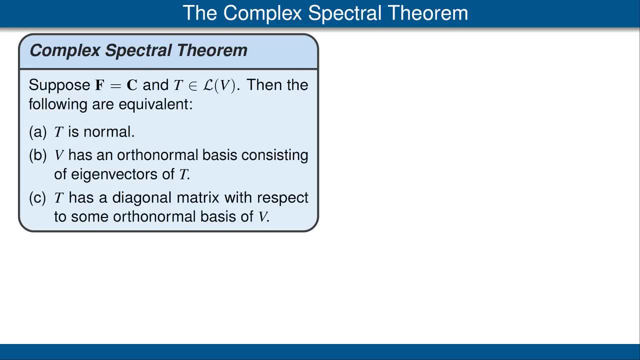 inner product space and an operator T on that inner product space, Then the following are equivalent. Condition A is that T is normal. Remember that normal means that T commutes with the adjoint T star. Condition B is that our inner product space V has an orthonormal. 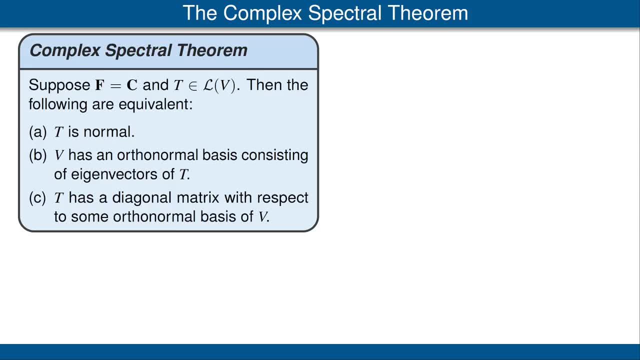 basis consisting of eigenvectors of T. Condition C is that T has a diagonal matrix with respect to some orthonormal basis of our inner product, space V. This is a marvelous theorem because it completely answers the question of which operators on a finite-dimensional, complex inner product. 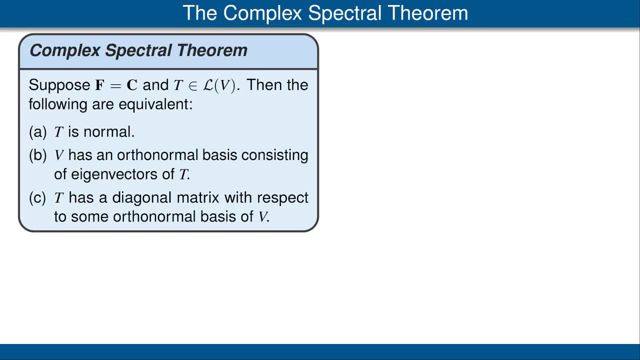 space have a diagonal matrix with respect to some orthonormal basis of the inner product space. Specifically, the operators with that property are precisely the normal operators. To prove the complex spectral theorem, we will start with the easy implications. Let's first suppose that C holds. In other words, we are 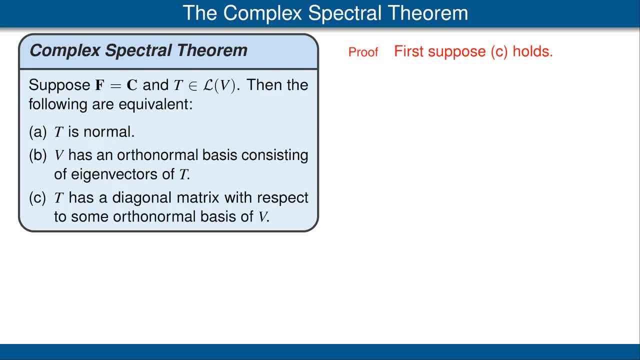 the T has a diagonal matrix. with respect to some orthonormal basis of V. The matrix of the adjoint T star is obtained by taking the conjugate transpose of the matrix of T. That's because we're using an orthonormal basis given by condition C. 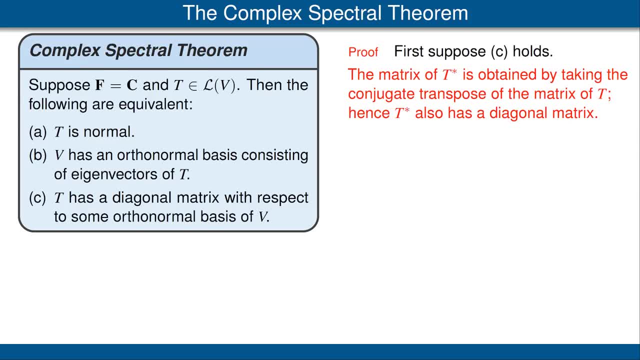 When we take the conjugate transpose of a diagonal matrix, we get another diagonal matrix, So T star has a diagonal matrix. It's easy to see that any two diagonal matrices commute under matrix multiplication. This allows us to conclude that T commutes with T star. 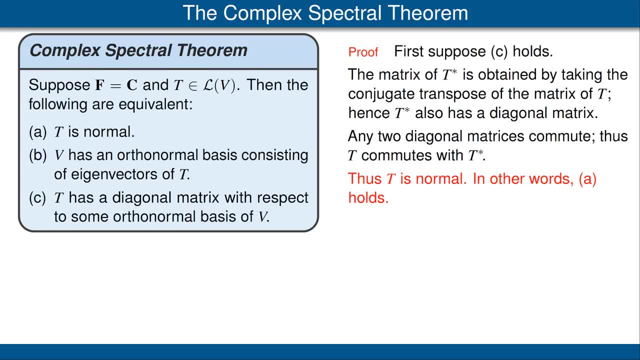 In other words, T is normal. Thus condition A holds. We have proved that condition C implies condition A. The equivalence of conditions B and C is very easy. We've discussed that previously, so there won't be any further discussion of that. 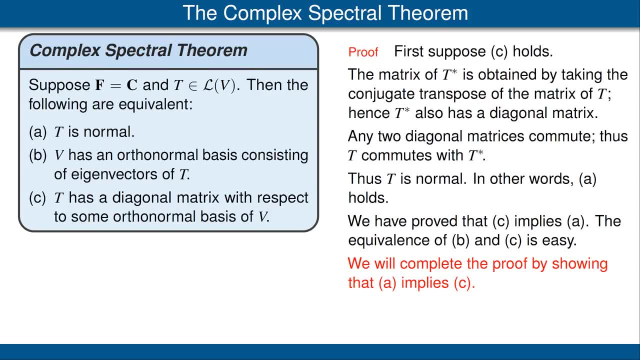 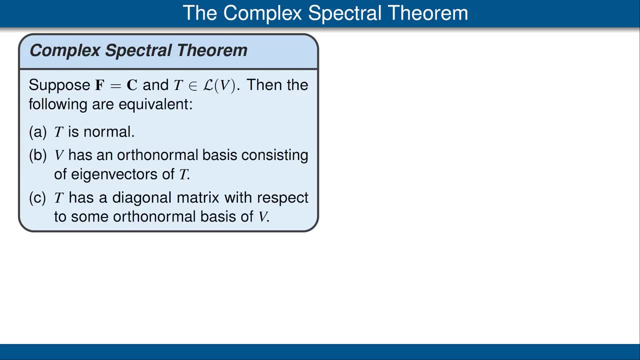 Now to complete the proof. we'll show that condition A implies condition C. To do that, we're going to have to wipe away the proof that's now visible. Now we want to prove the harder part of the spectral theorem. In other words, we will show that A implies C. 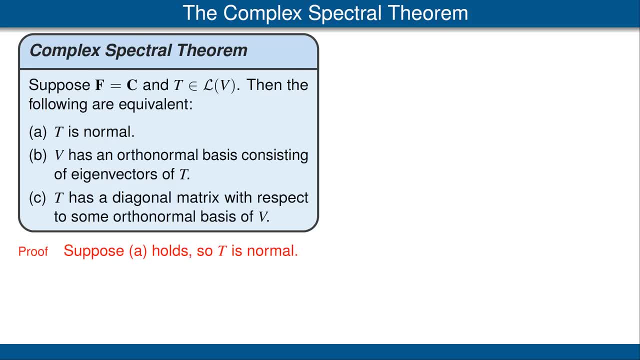 Suppose A holds, so T is a normal operator. on V We call Shur's theorem. It says that in a complex finite system, given any operator, there's an orthonormal basis with respect to which that operator has an upper triangular matrix. 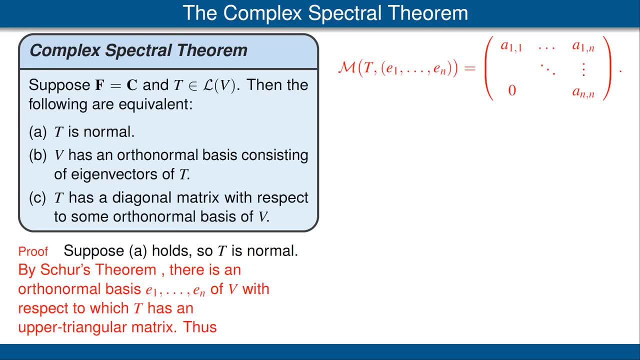 This is where we're using the hypothesis that our scalar field is the complexes. Thus we have an orthonormal basis- E1 up to En of V, such that the matrix of T with respect to that basis is as shown in the second column. 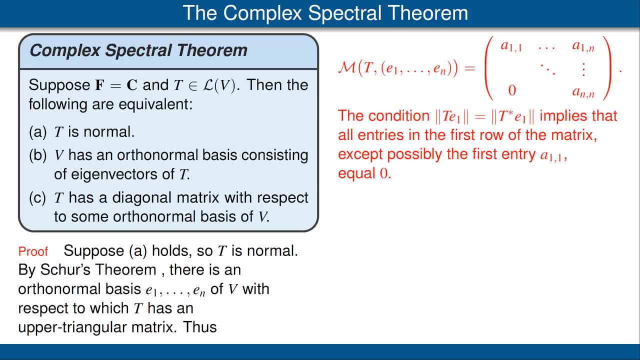 namely an upper triangular matrix. Because T is normal, the norm of T applied to any vector is equal to the norm of T-star applied to that same vector, as we showed in a previous video. Let's apply that result to the vector E1, our first basis vector. 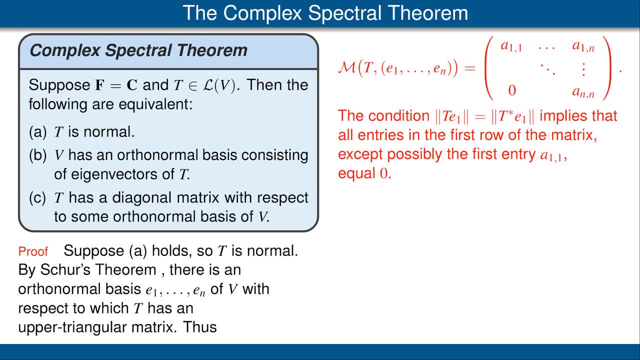 so we know that the norm of T of E1 is equal to the norm of T-star of E1.. The norm squared of T of E1 is equal to the sum of the squares of the absolute values of the vector E1.. The norm squared of T of E1 is equal to the sum of the squares of the absolute values of the first row of the matrix shown above. 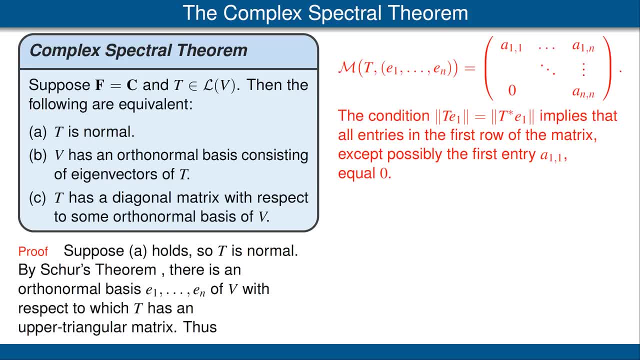 Because of the upper triangular form, that's equal to the absolute value of A11 squared. The matrix of the adjoint of T is obtained by interchanging the rows in the columns of the matrix of T and then taking complex conjugates. Thus the norm squared of T-star of E1. 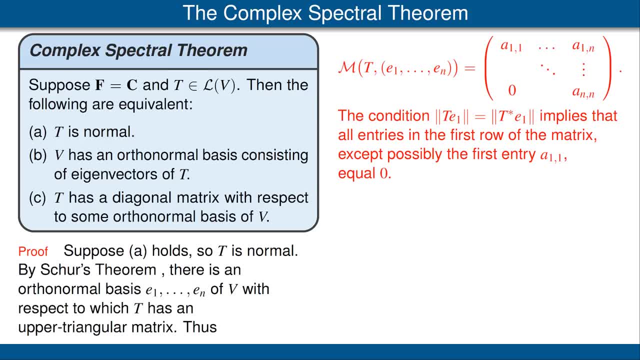 is equal to the sum of the squares of the absolute values of the first row of the matrix shown above. Thus, this equality of norms implies that all the entries in the first row of the matrix, except possibly the first entry, A11, equals zero. 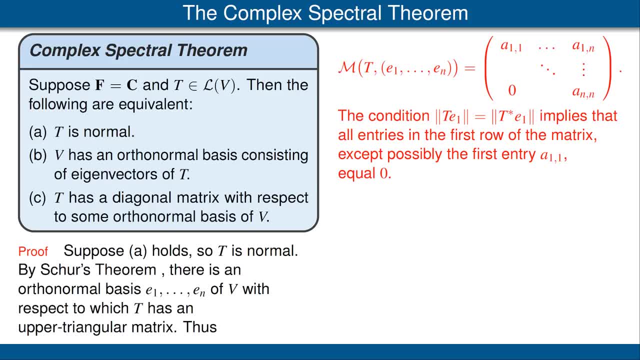 You should pause the video and make sure you understand this crucial point. If necessary, look at the details in the book. Now let's look at the equation. the norm of T of E2 is equal to the norm of the adjoint of T applied to E2.. 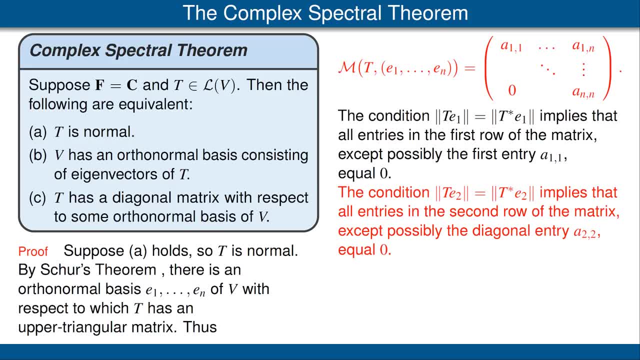 Again, we can compute these norms, or at least the norm squared coefficients, in the matrix. We already know that the first row of the matrix is 0, except for, possibly, the entry A11.. And now, when we think about this new condition that we're 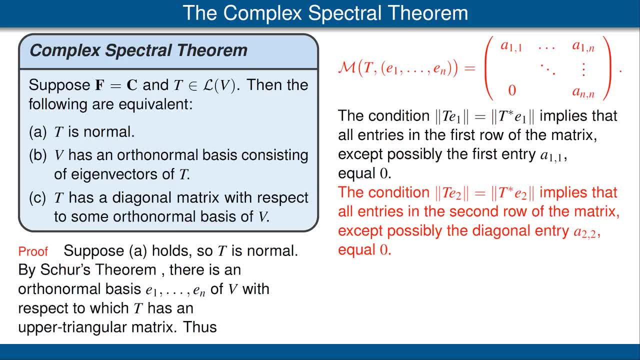 considering this shows that all the entries in the second row of the matrix, except possibly the diagonal entry A22, are also equal to 0.. Continuing in this fashion, we see that all the non-diagonal entries in the matrix equal 0.. Thus, the matrix above is a diagonal. 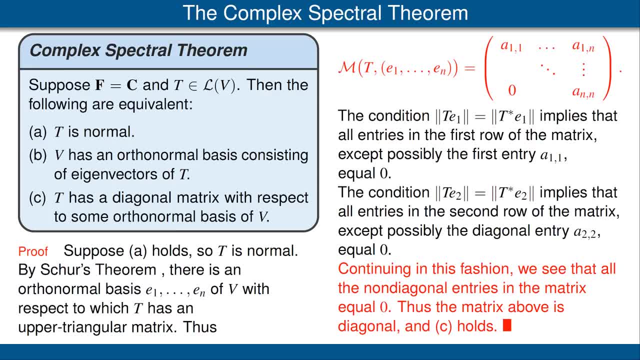 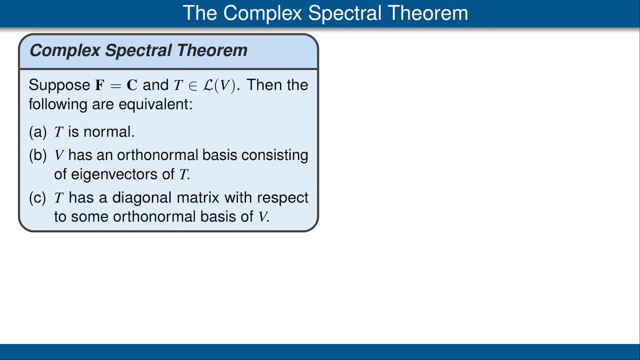 matrix, In other words, condition C holds. This completes the proof of the complex spectral theorem. Let's look at an example of the complex spectral theorem which is stated here in the first column. Consider the normal operator T on C2, whose matrix is the matrix shown here. 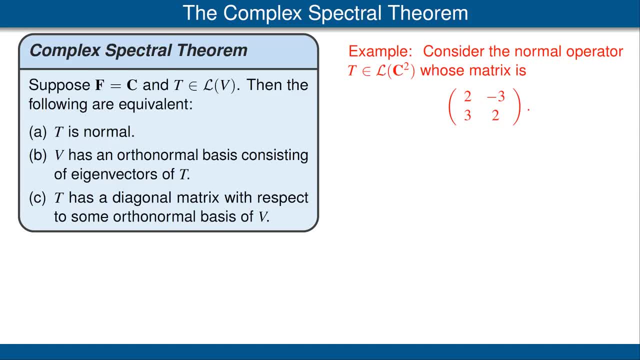 Of course we're using the standard inner product on C2 and the standard orthonormal basis. We verified in a previous video that this operator T is indeed normal. As you can verify, the list of two vectors shown here is an orthonormal basis of C2 consisting of: 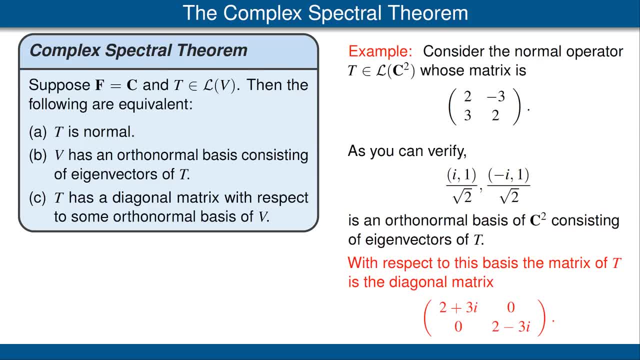 eigenvectors of T With respect to this basis. the matrix of T is the diagonal matrix shown here. Thus, by choosing the correct basis, we changed the matrix so that it has zeros off the diagonal. That's not such a big deal for a 2x2 matrix, but if we were dealing with a larger matrix, 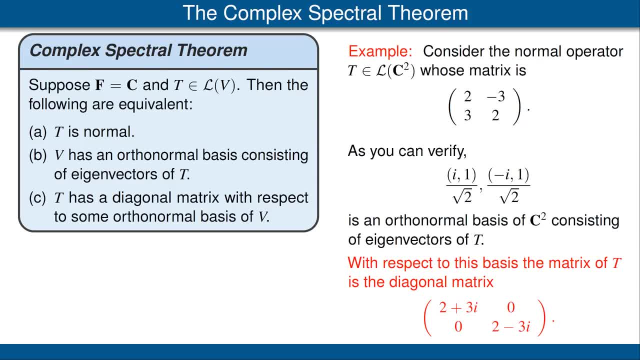 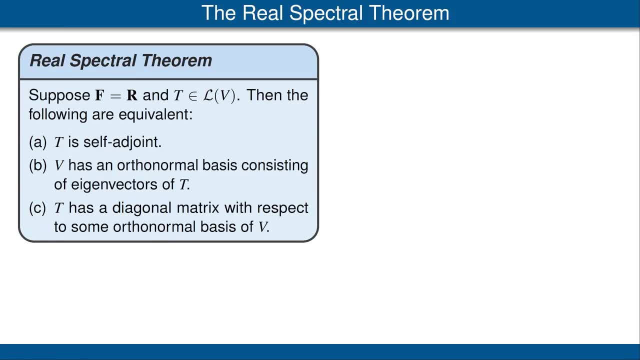 that would be a huge improvement and a huge simplification. We now turn to the real spectral theorem. The real spectral theorem says that if we have a finite-dimensional real inner product space and an operator T, we have a finite-dimensional real inner product space and an operator. 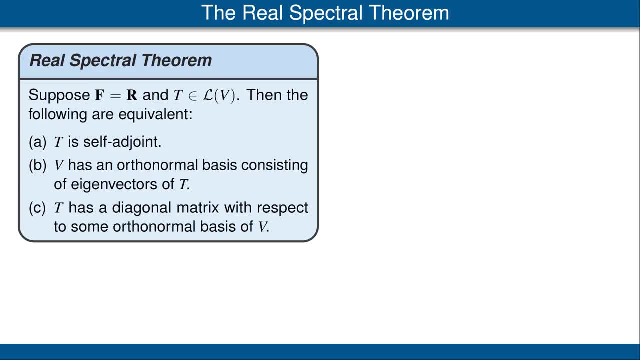 T- we have a finite-dimensional real inner product space and an operator T- we have a finite-dimensional real inner product space. then the following are equivalent: Condition A is that T is self-adjoint. Condition B is that V has an orthonormal basis consisting. 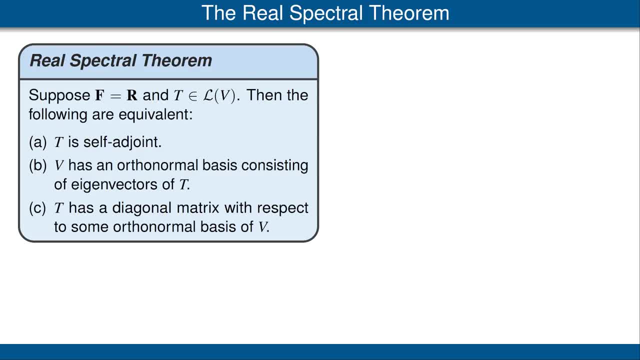 of eigenvectors of T. Condition C is that T has a diagonal matrix with respect to some orthonormal basis of our inner product space V. Conditions B and C are the same as for the complex spectral theorem, but Condition A is different.